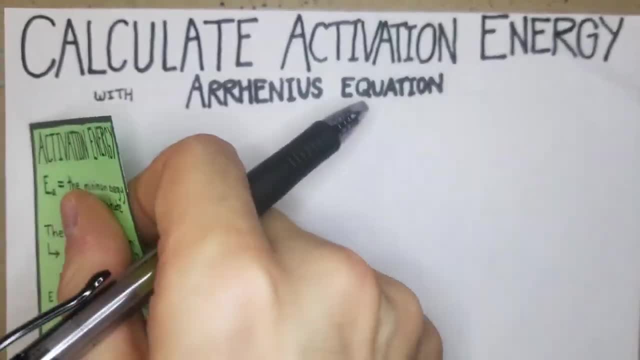 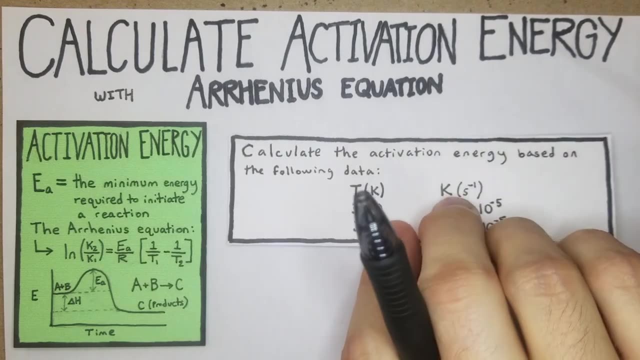 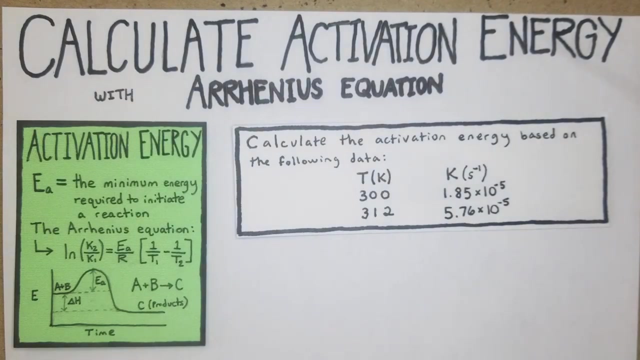 the end. So with that out of the way, we will jump into the first problem I have. So calculate the activation energy based on the following data: we have 300 and 312 and that's in Kelvin. and for our K values we have 1.85 times 10 to the. 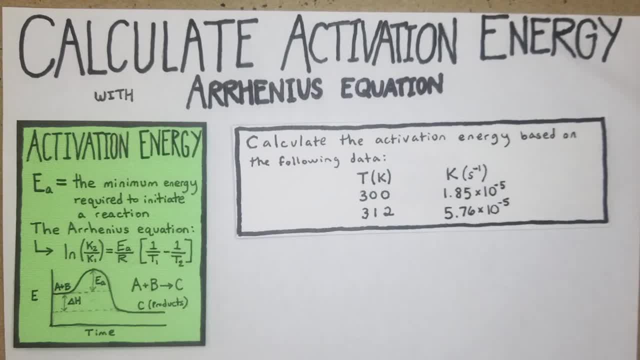 negative 5th and 5.76 times 10 to the negative 5th. so we're just going to plug that right into the equation. what we have here, so the natural log, we're going to do K2 over K1. I'm going to take 5.76 times 10 to the negative 5. that's going. 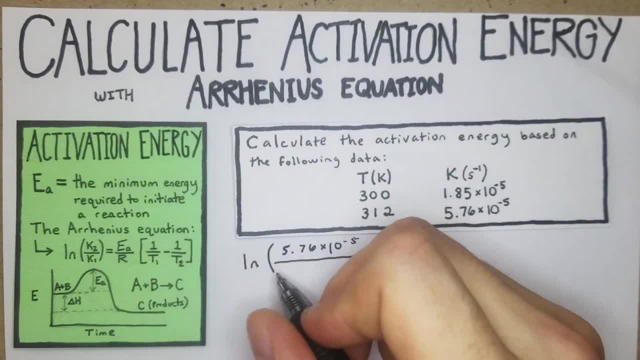 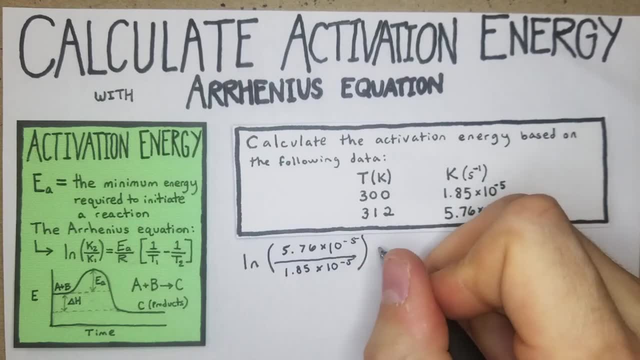 to be divided by our K1 value, which is going to be 1.85 times 10, to the negative 5th. so you have the natural log of that. that's going to equal the EEA over 8.31 joules per mole Kelvin, and that's going to be our R value. and then 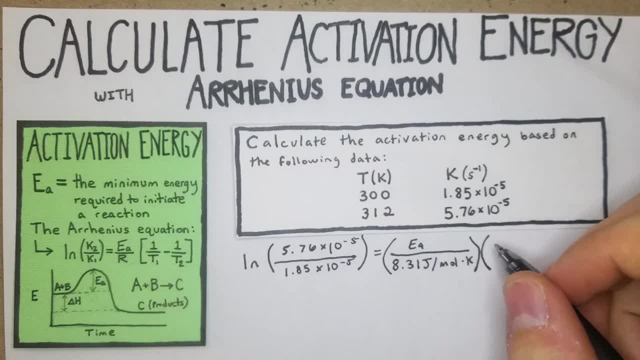 what we have is our 1 over T1 minus 1 over T2, and our K1 should correlate to our T1 and our K2 should correlate to our T2. so here what we're going to have is our 1 over T1, which in this case will be the 300 K, and then minus 1 over our 312. 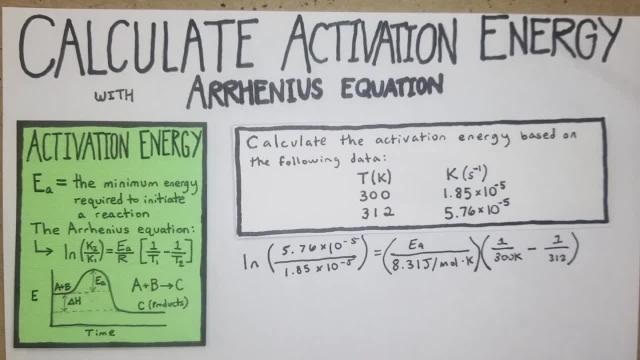 and then we're just going to solve that. so because there's no variables on the side, that makes it pretty convenient because the natural logs, there be a little bit more work to get rid of that later. but here we have 1.1358, it's going. 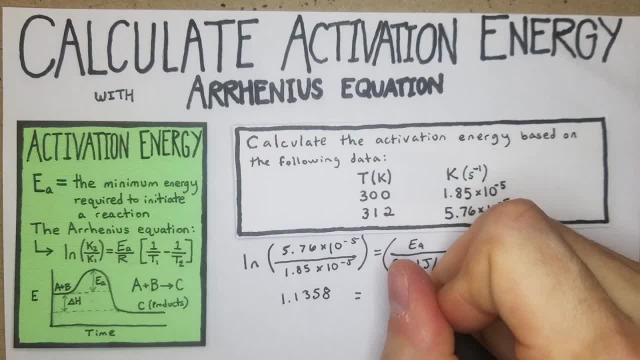 to equal our EA over 8.31 joules per mole times, Kelvin times, I'm getting a really small 0.001285,. so we're going to say 1.28 times 10. to the negative fourth we'll say: and that's this value here. 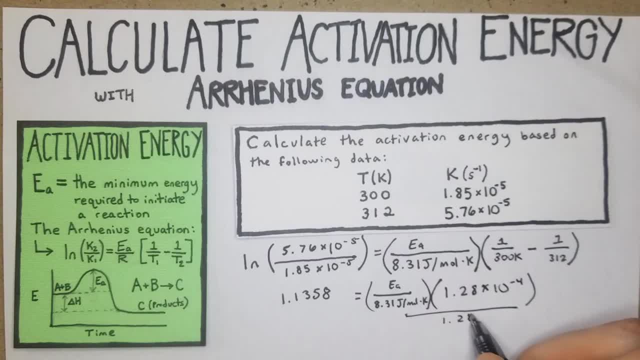 So now what we can do is we can divide both sides by 1.28 times 10 to the negative fourth. divide this side by the same 1.28 to the negative fourth. So now we're going to do that out. 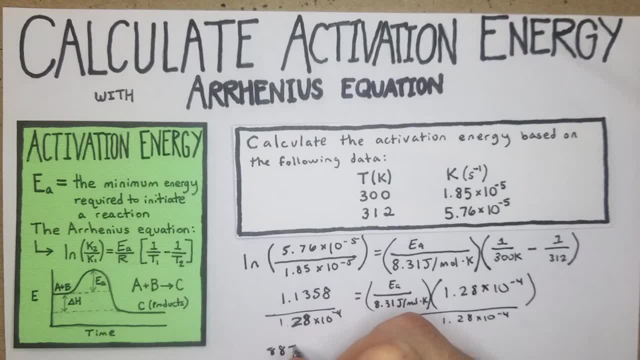 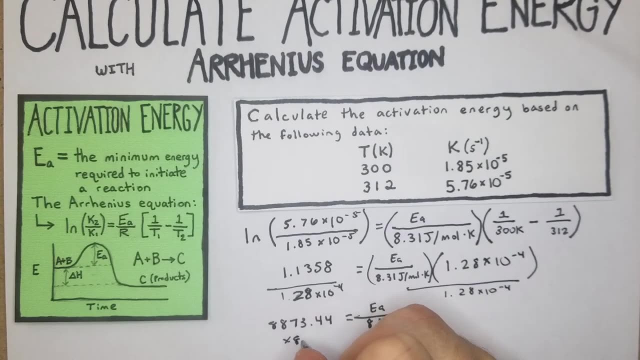 So here I'm getting. 8.873.44 is equal to the Ea, the activation energy, over 8.31.. So we can multiply both sides by 8.31.. Okay, Our activation energy is going to be: we've got 73738.2657,. we'll say we'll round and 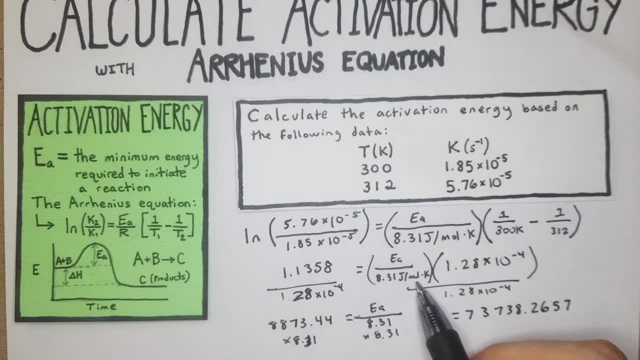 then what we can, and that's going to be. we'll look back at our units. We have joules, We have joules, We have joules per mole times, Kelvin, here and then here we have our values, our K values. 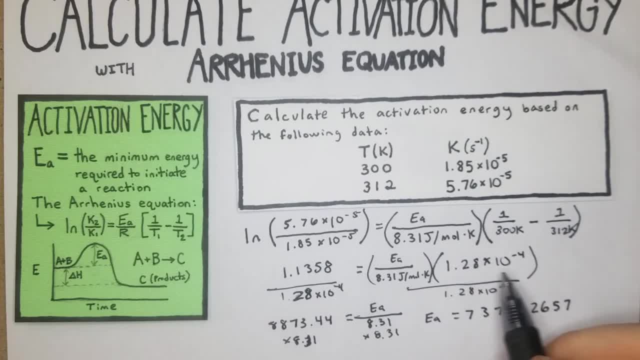 So we got rid of K because K was on the bottom, and we multiplied it by K and we got: we have moles on the bottom, we have joules on top. What we're going to end up with here from these calculations is joules per mole, because over 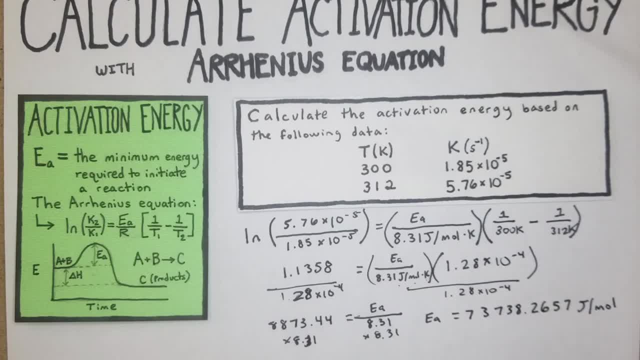 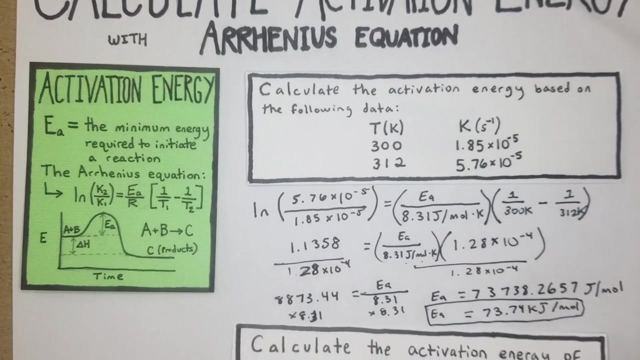 here it's joules per mole times Kelvin. we got rid of Kelvin joules per mole And then we can say our Ea is going to equal 73.74 kilojoules per mole. So there's our first one, And then we'll just move down, jump into the second- one kind of overlap, this just so we. 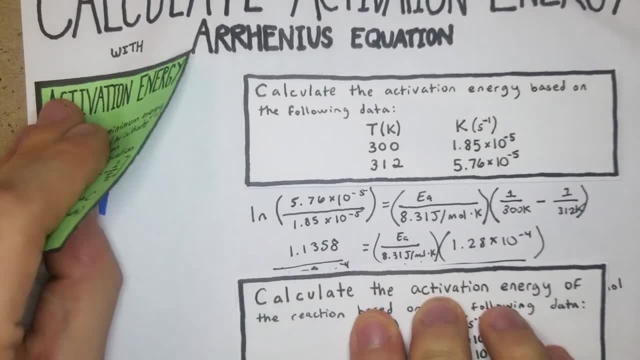 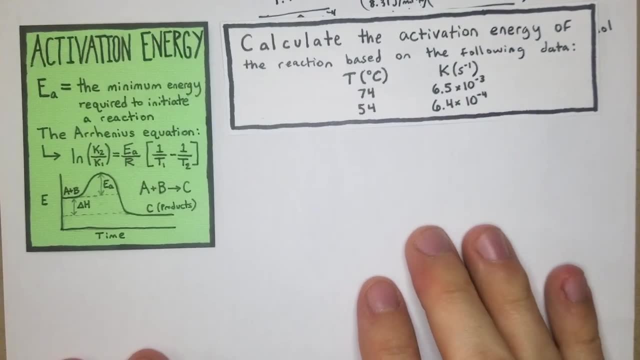 can get a little extra space, Okay, And then we'll just move down, We'll just drop this down, Okay. So this is going to be our Ea, All right, So calculate the activation energy of the reaction based on the following data and: 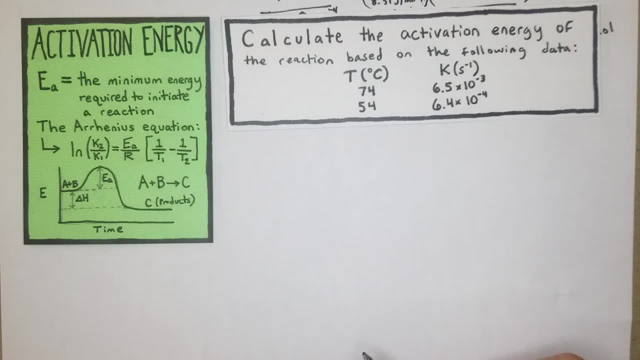 we have some points there. So first of all, just like we did in the last problem, what we're going to start with is our equation. We have the natural log of our K2 over K1.. We'll do the 6.4 times 10 to negative 4.. 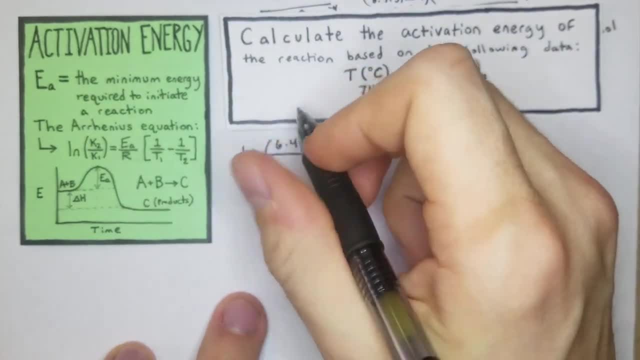 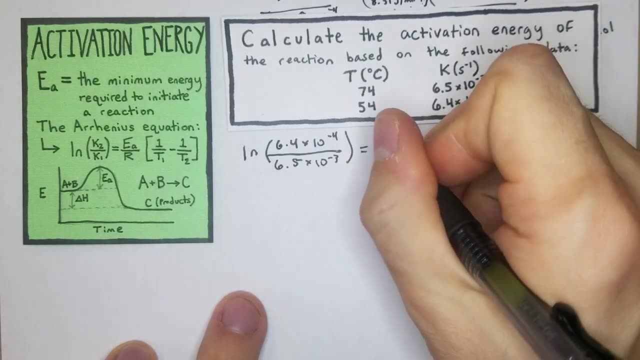 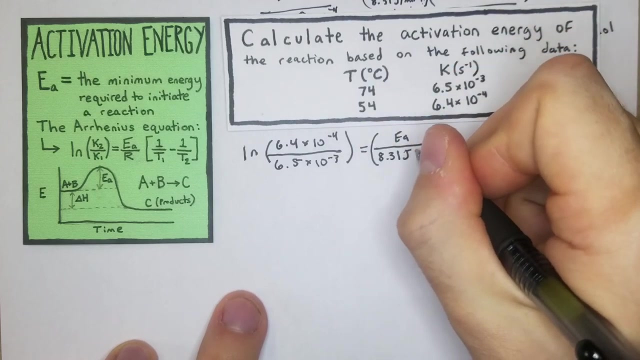 And that's going to be over K2.. So that's going to be over K1.. Okay, over our 6.5 times 10 to the negative 3 set that equal to EA over 8.31 again, while you were using that same value, Joules per mole times Kelvin, and then. 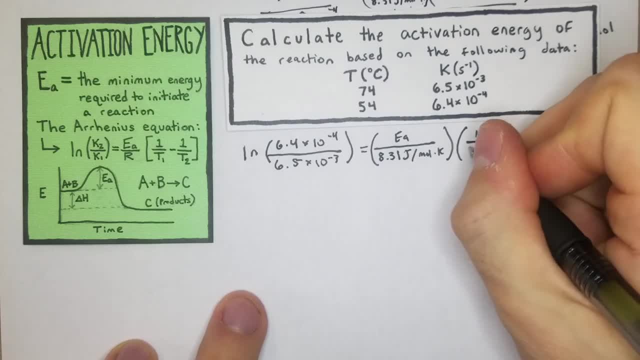 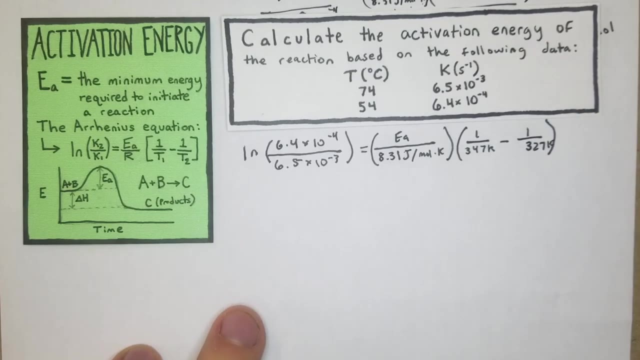 our t1, which in this case is going to be 347 Kelvin. that's after we add 273 to each one, and then over here we have 1 over 327 Kelvin. so now we've got some math to do. I like figuring out everything that we can first, I mean. 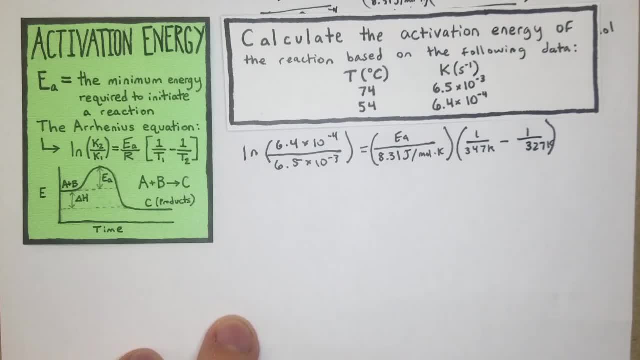 obviously we'll start with this and this and then we'll work from there to solve EA. so what I'm gonna get for this value over here: zero point, zero point, zero point, zero, zero, zero. one seven, six, two, six Kelvin- it's obviously a very small number, that's negative. and then times the EA over 8.31 is equal to, and then 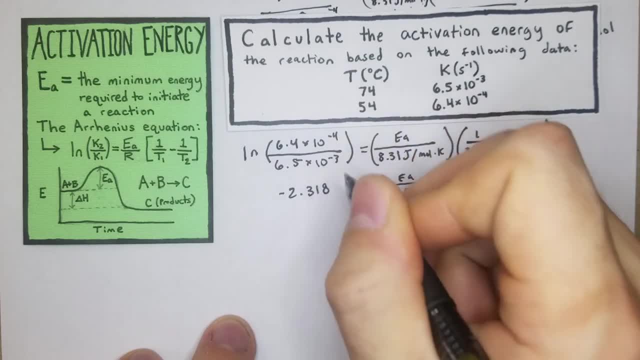 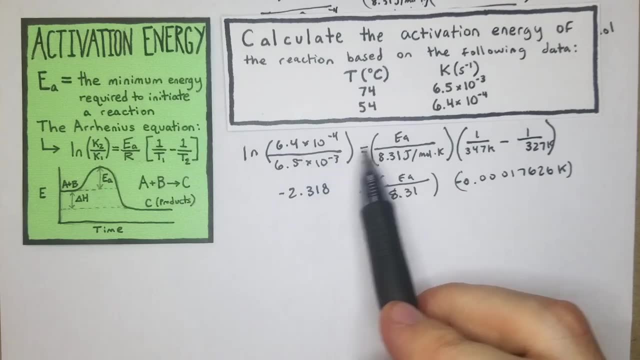 here we get a negative 2.318. so in this case, what we did is our, our K2 and our T2 were the, the, the second values of the lower of the two, and in the previous one they were the higher of the two, and in this case, what we're 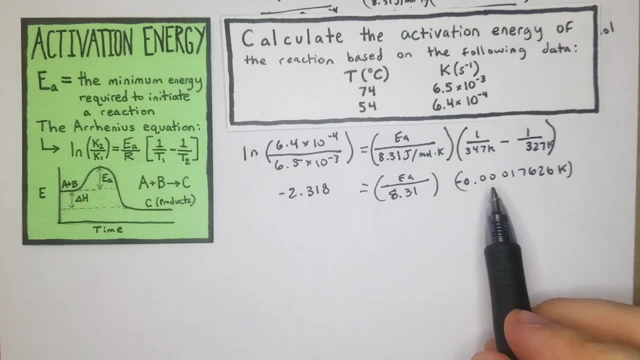 going to find out here is we get a negative number on both sides. so it's going to end up, you know, it's going to end up working out in the end just the same as if we had swapped the values. so we're gonna do is divide both sides by. 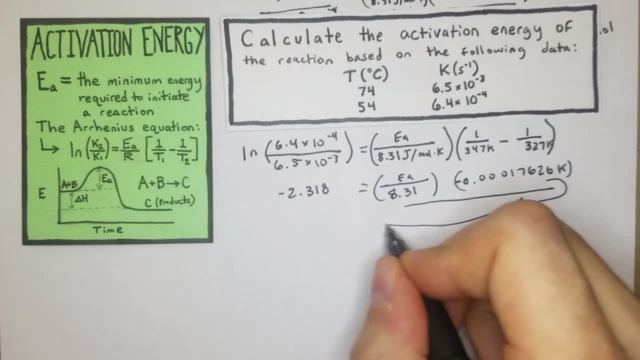 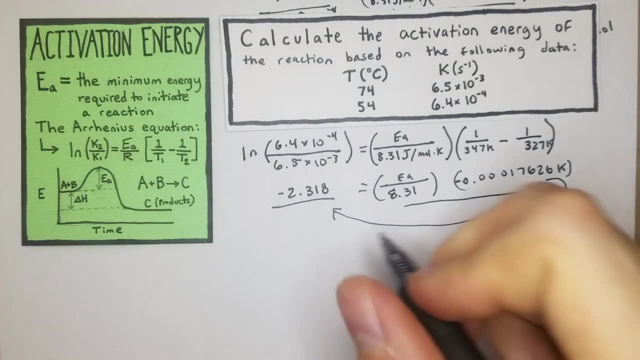 this you, and what we're gonna get in is one three, one, five one point. oh three is equal to our EA over eight point three one. and I like ending with this step every time when I can, just cuz you know it's consistent: eight point three, one. so 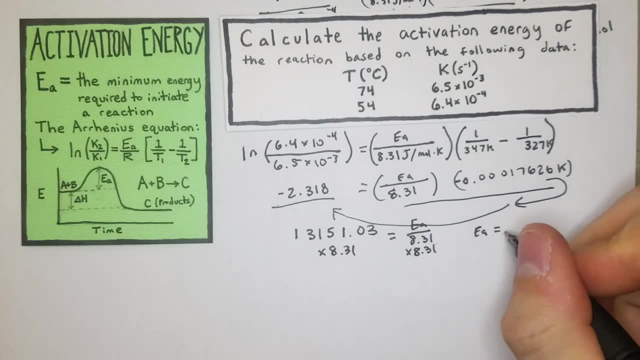 our EA. it's going to equal one zero nine. eight point three, one. so our EA is going to equal one zero nine, two, three, 285, and again what we have is Our joules per mole times Kelvin. we get rid of Kelvin, We're left with joules per mole and 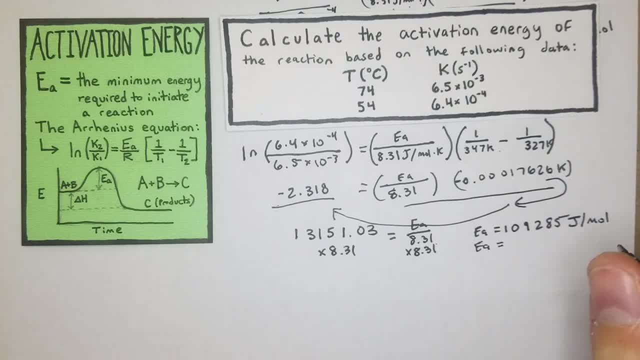 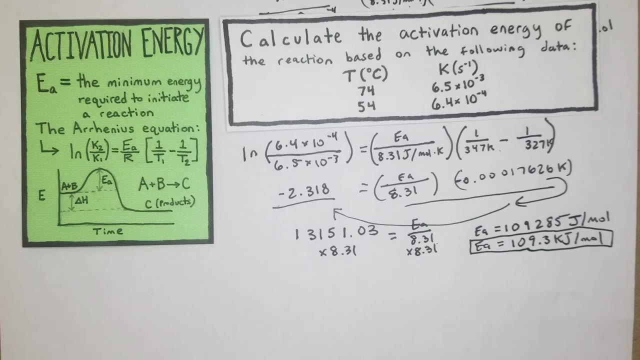 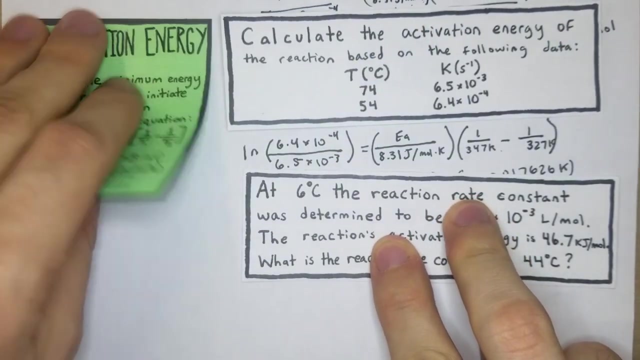 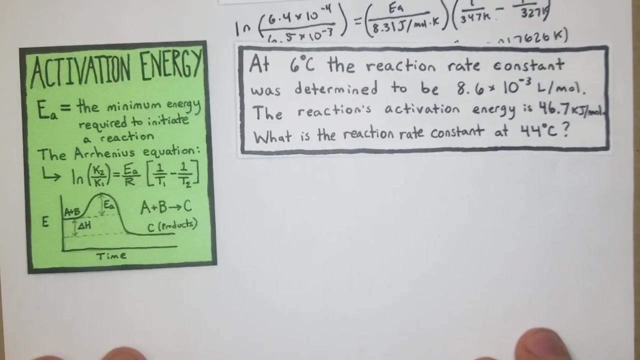 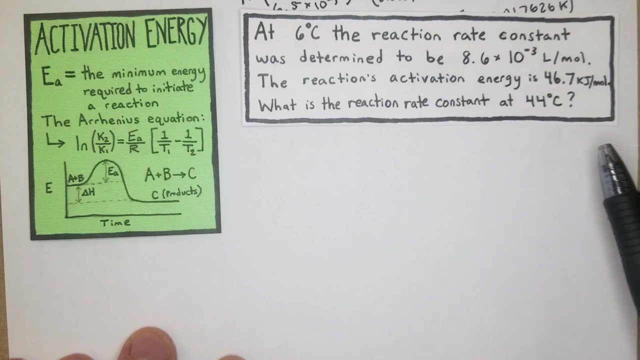 Then what we can say is: our ea is going to equal 109.3 kilojoules per mole. All right, so now we can move on to our third and final problem in this set. There we go, All right. at 6 degrees Celsius, the reaction rate constant was determined to be 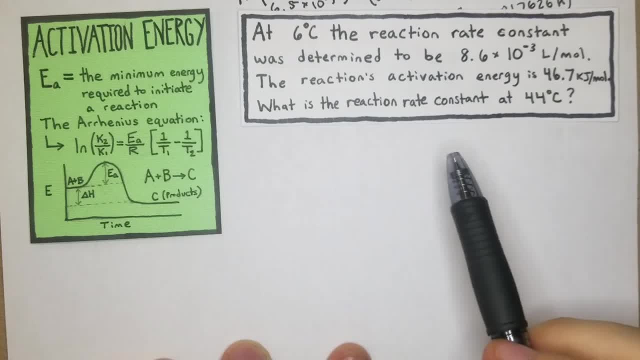 8.6 times 10 to the negative 3 liters per mole. so the reactions activation energy is 46.7 kilojoules per mole. What is the reaction rate at 44 degrees Celsius? So, like I said in the beginning, with the Arrhenius equation, 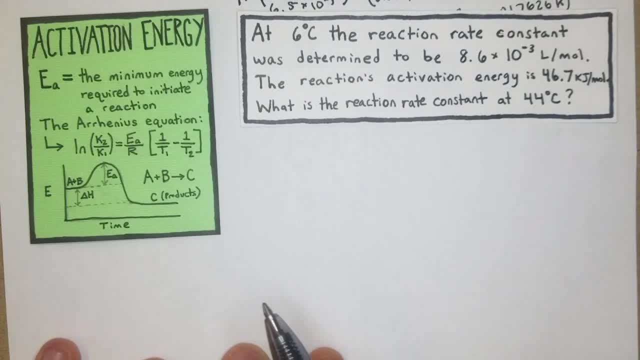 What's kind of cool about it is, if you have the K value at two different, I'm sorry. If you have the K value at one temperature and the activation energy, you can calculate K at any other temperature. and now it's giving Us another temperature that we can use in this equation to calculate, So we're gonna have this. 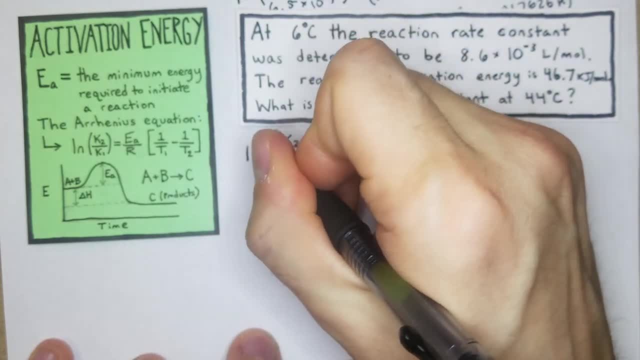 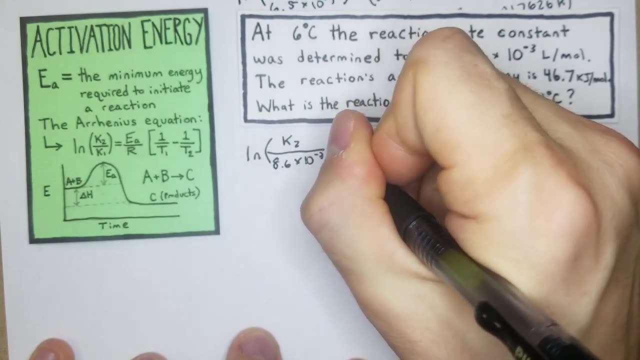 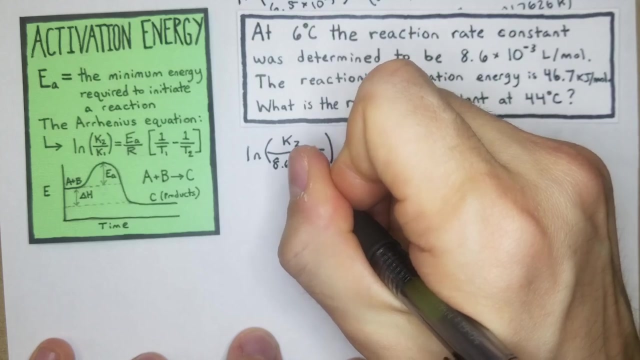 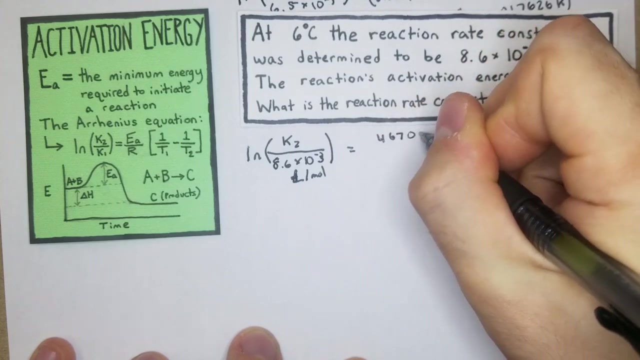 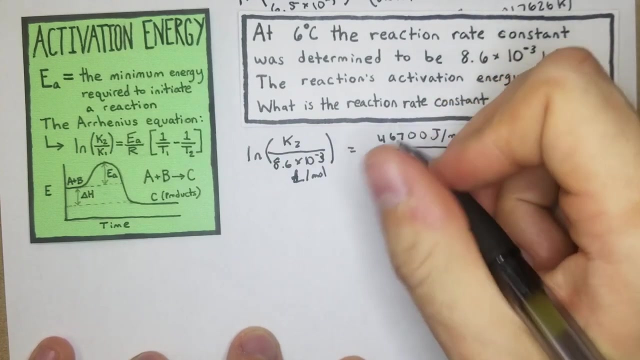 natural log of K2 Over 8.6 times 10 to the negative 3, and That's going to be in the liters, I'm sorry, L per mole And that's going to equal four, six, seven, oh, oh, joules per mole. and the reason that we're putting that into joules is because our R value is already in joules. 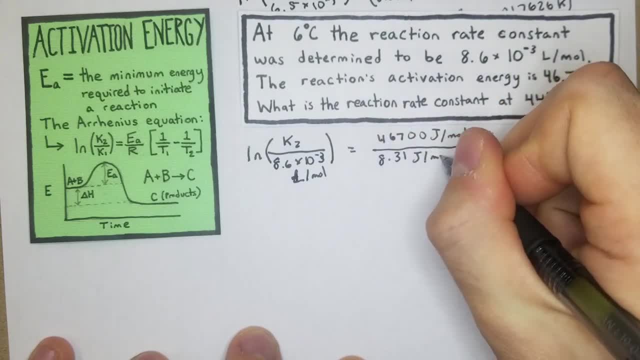 So we're going to use that same 8.31 joules per mole times K And now you can see if we're solving for a different variable we're going to end up with. you know we're gonna get the units that that You know for K rather than the units for T like we did in the last two. I'm sorry for the yeah. 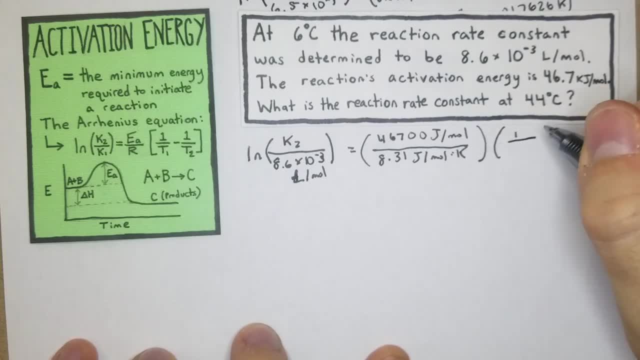 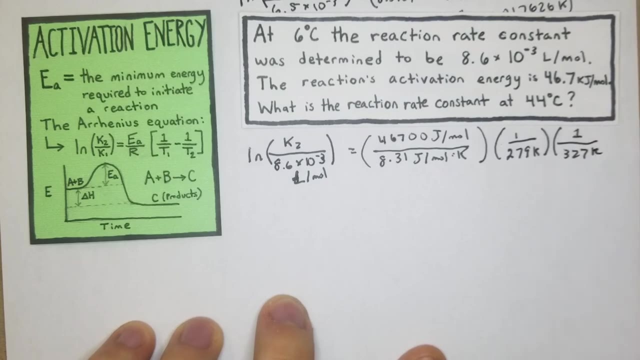 So here we go now. we have one over What's gonna be our. So our T1 value is going to be 279. Okay, Kind of wrote it a little weird there, but I think it'll be okay. ok, and then we'll just double bracket that put a minus sign in between there. 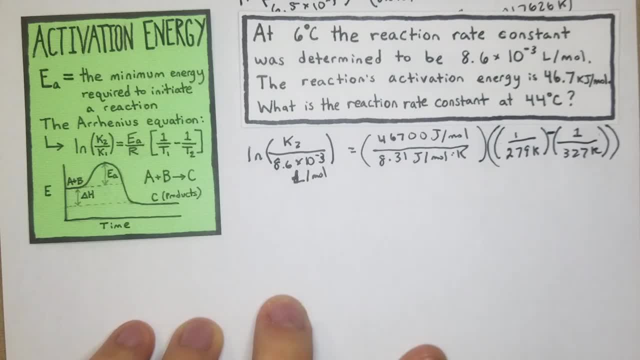 All right, and now we can start solving. So in this case we can't start with the natural log like we did in the previous one, so we're going to have a different type of step for solving that, but we can work from the middle. 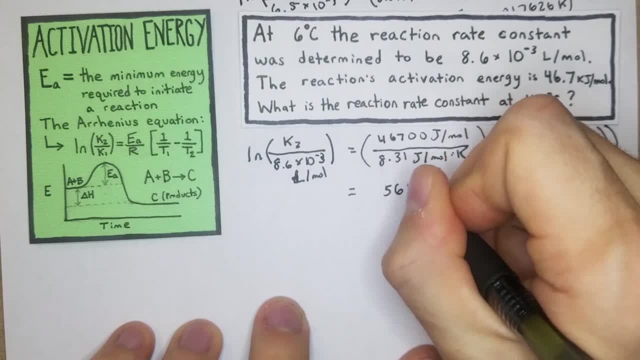 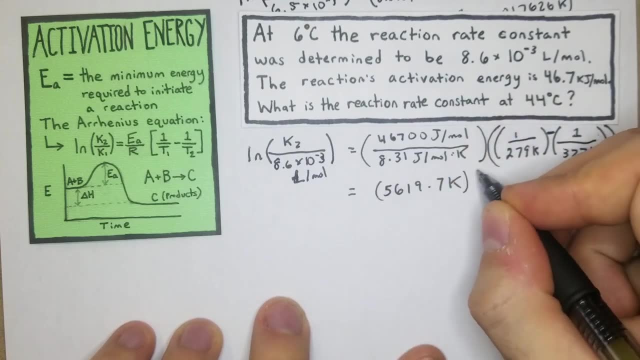 So we have 5,, 6,, 1,, 9,, 0.7, K, because we have joules per mole, joules per mole left with just K, And then over here we're going to get 4.2966 times 10 to the negative 4.. 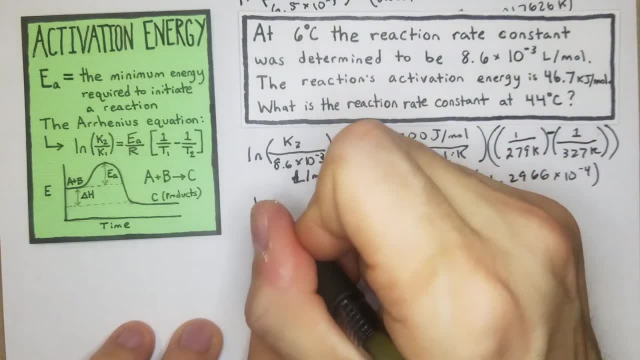 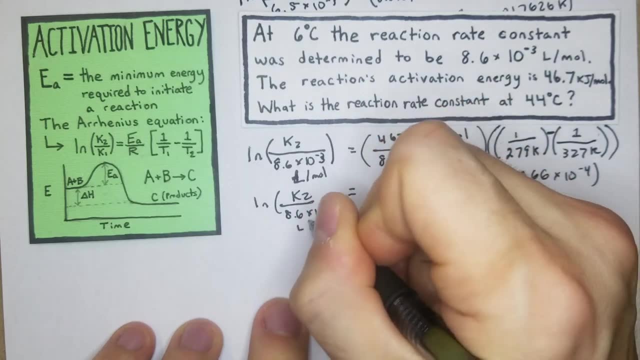 And then we're going to multiply that out. This is all equal to K2 over 8.6 times 10 to the negative 3, L per mole. So we're going to get here K2 over 8.6 times 10 to the negative 3, L per mole. 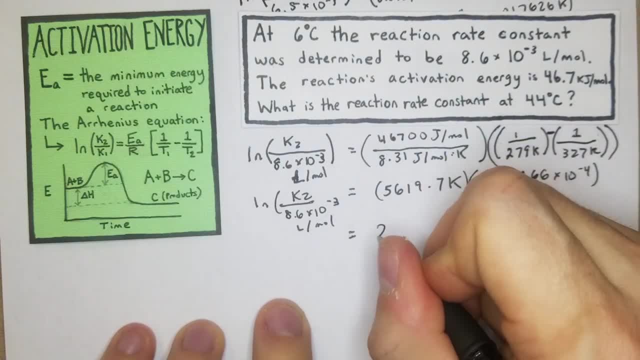 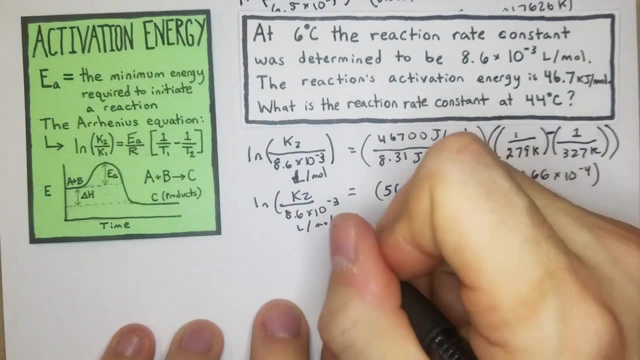 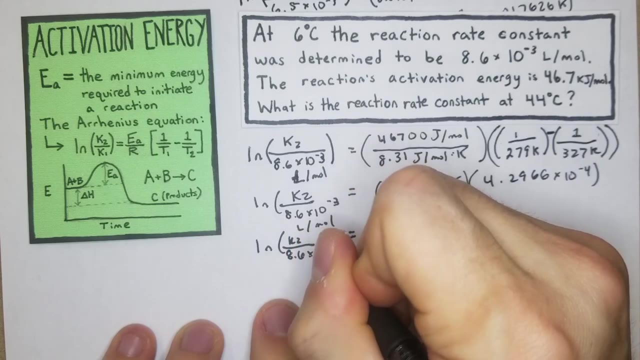 It's going to equal 2.4146.. Natural log of K2 over 8.6 times 10 to the negative 3.. So what we're going to do to resolve this? the first thing that we're trying to get rid of is the natural log here. 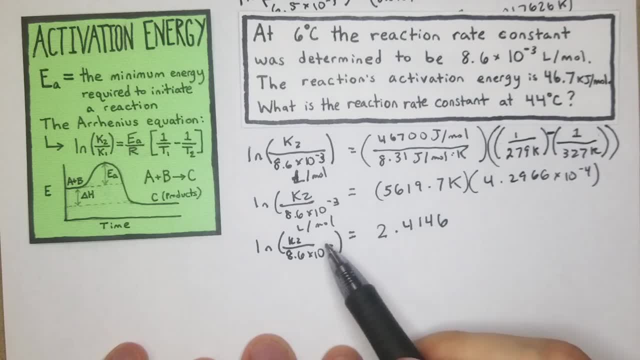 And we have a whole number. you know, we have a number and we have a log with the variable on it. What we're going to have to do is we're going to raise both sides to the E, So we have E natural log of K2 over 8.6 times 10 to the negative 3. 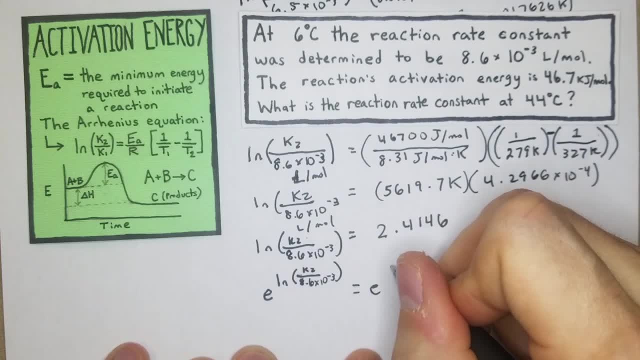 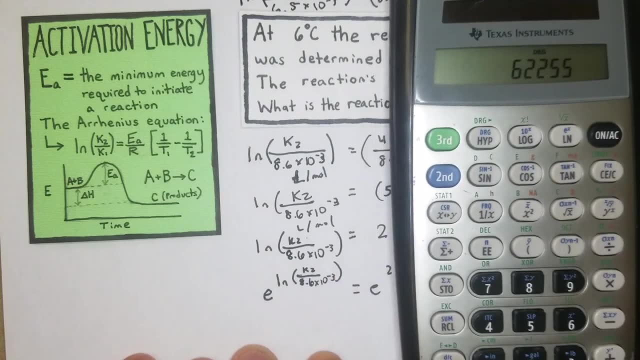 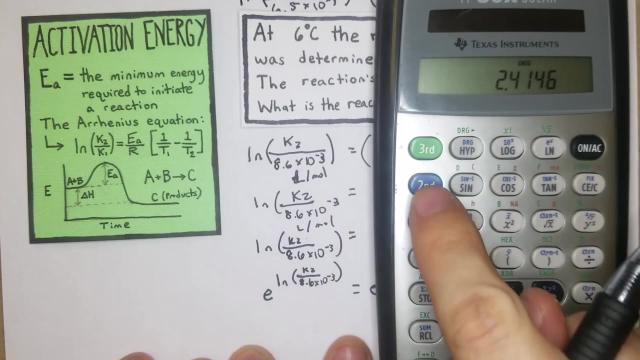 is equal to the E of 2.4146.. And the way I do that everyone's calculator is different, but my calculator here it's going to be so 2.4146.. And then I hit the second and then I have this E here. E to the X. 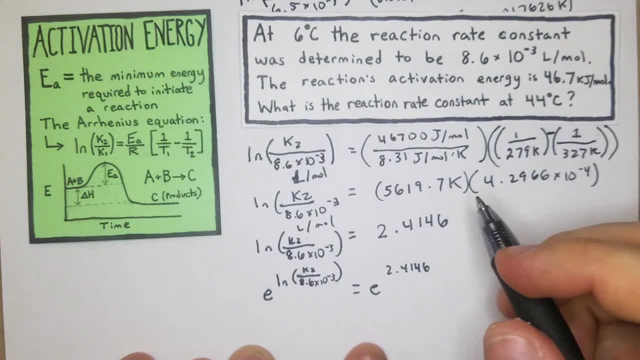 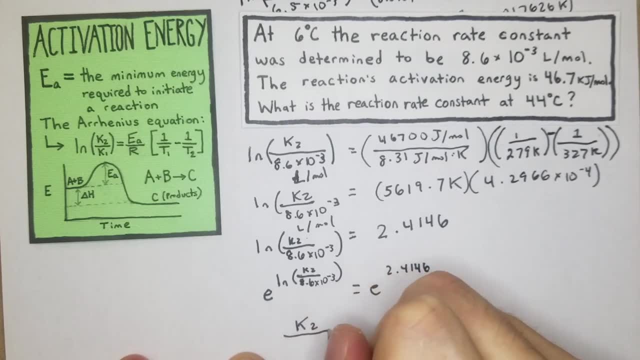 That's what I'm going to get for that. So here now I have K2, we got rid of the natural log. 8.6 times 10 to the negative 3, L per mole is going to equal 11.19.. 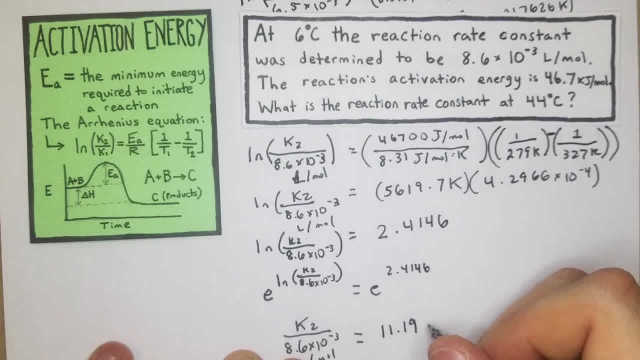 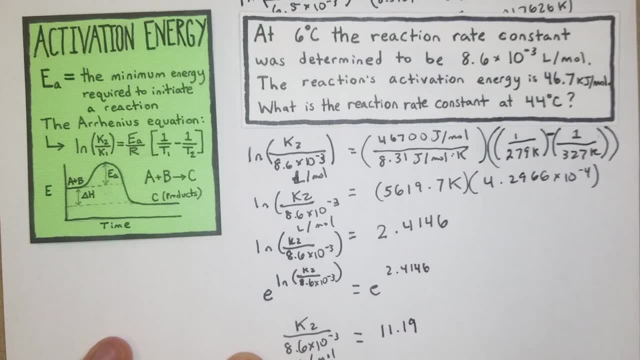 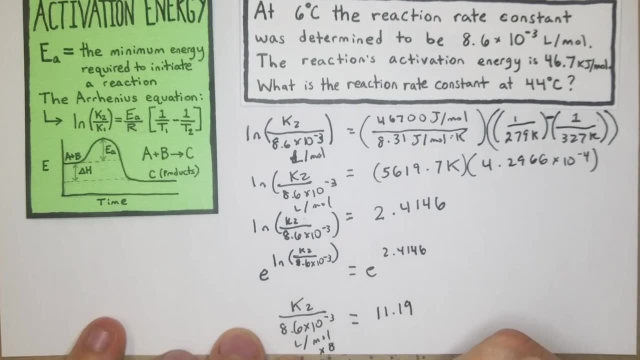 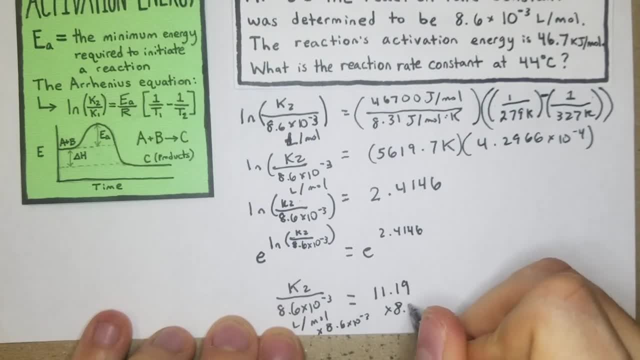 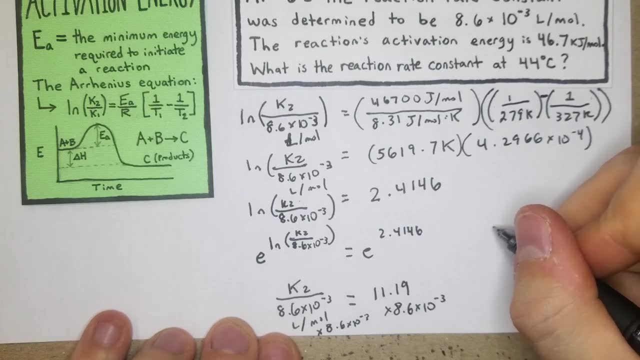 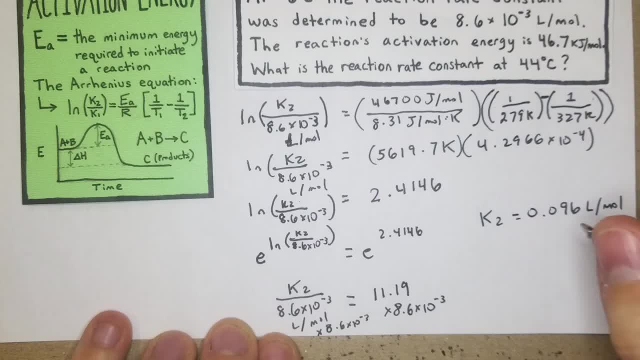 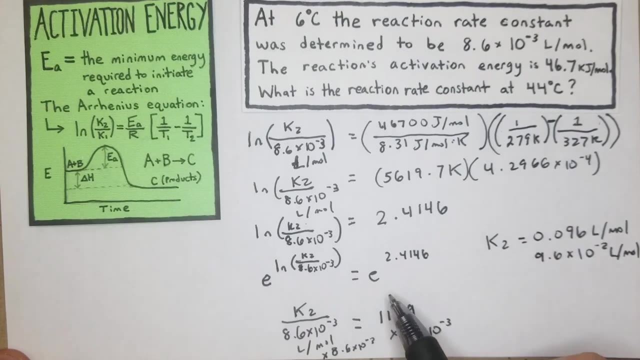 Okay, Okay, Okay. Or we can say it's 9.6 times 10 to the negative 2. L per mole. Now the thing with these calculations are there's like one other, I don't know if it's really a shortcut, but another way that I think is useful to conceptualize it. 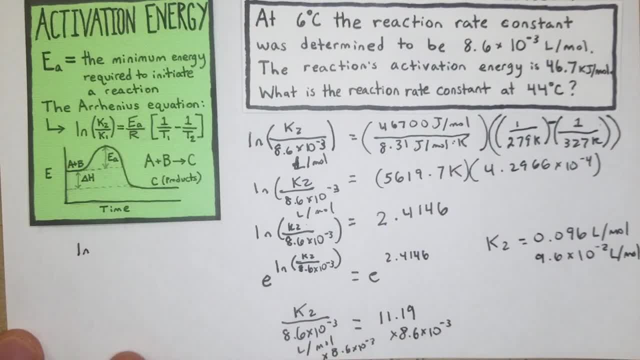 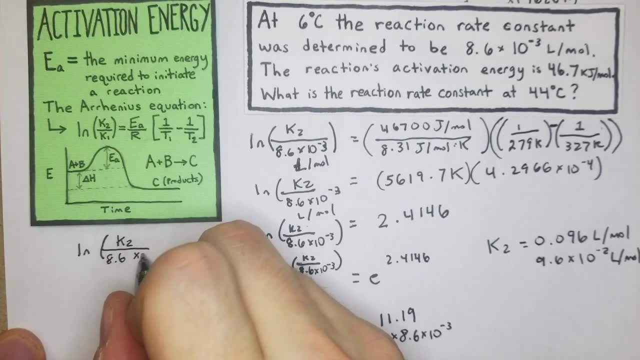 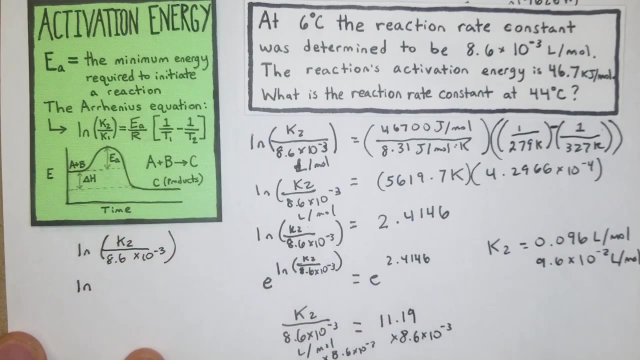 Like, for instance, over here you have the natural log: of K2 over 8.6 times 10 to the negative 2.. Okay, native 3.. Another way that that can be written, though, is like this: The natural.